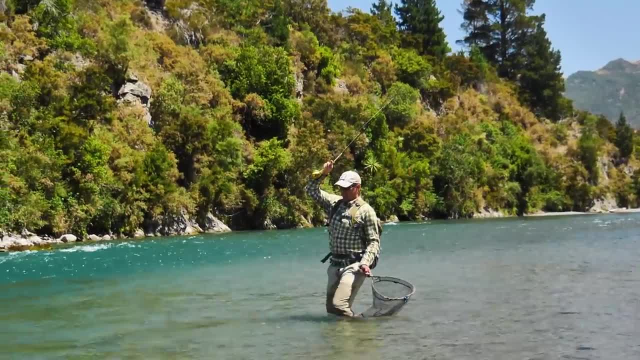 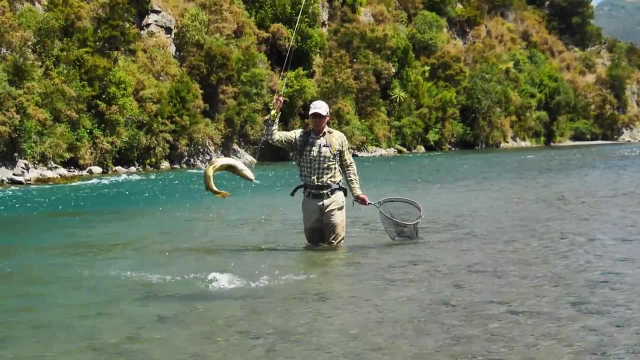 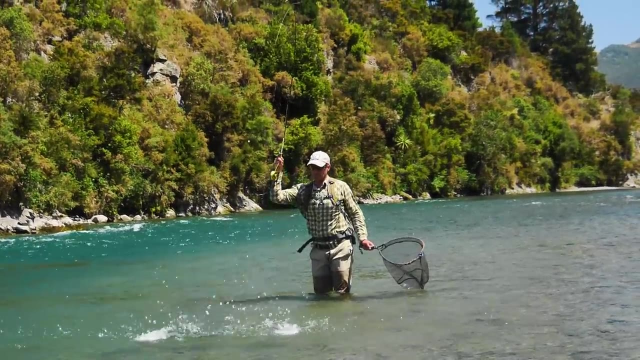 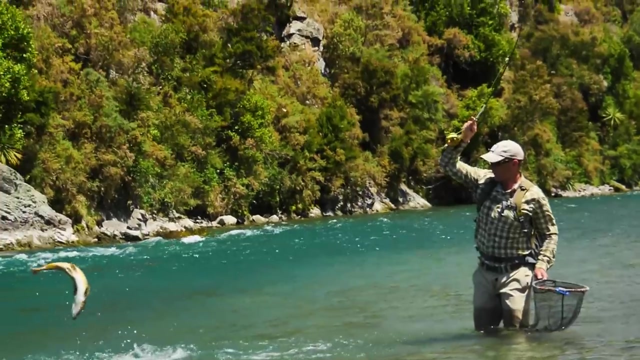 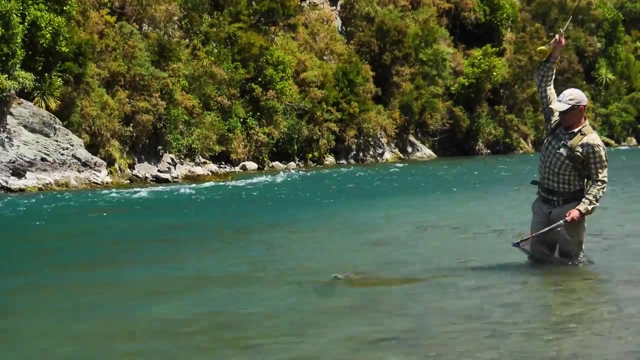 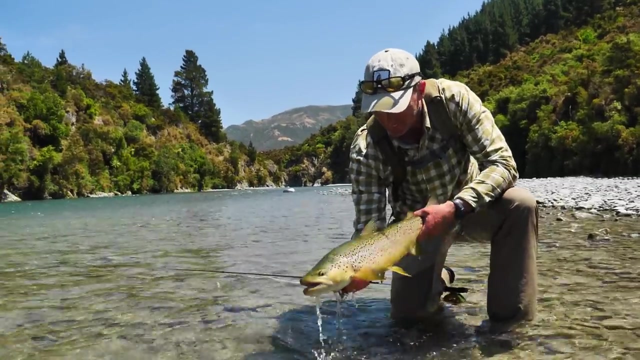 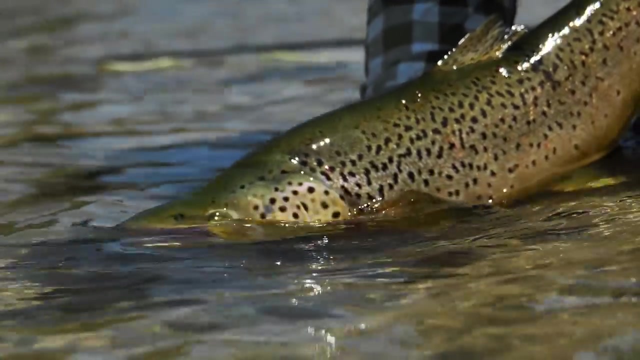 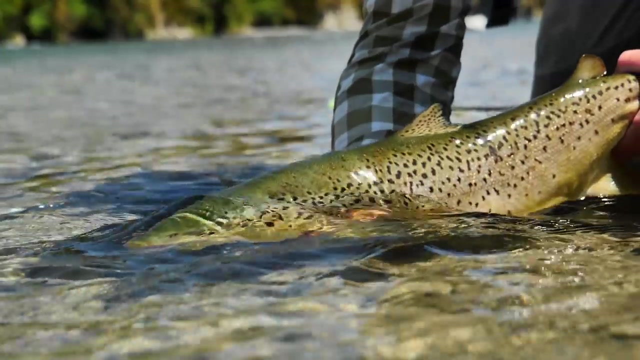 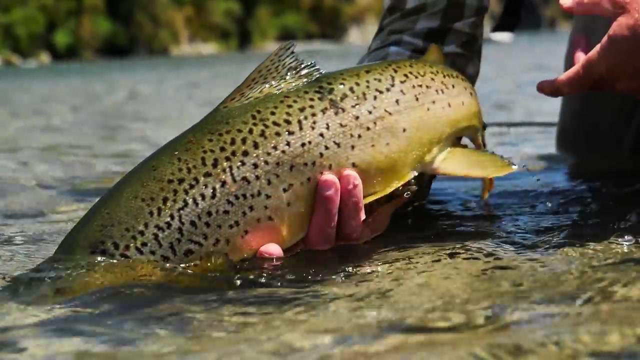 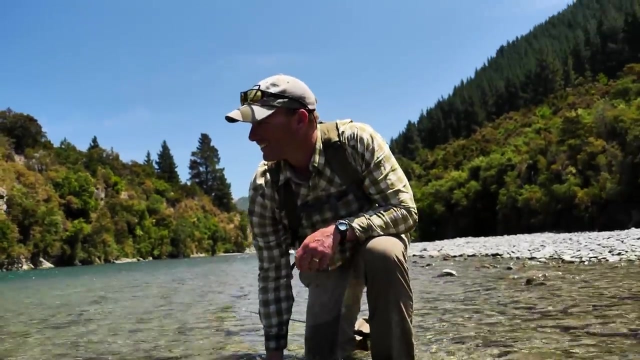 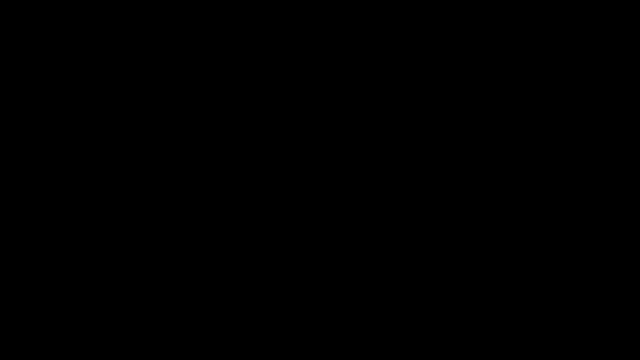 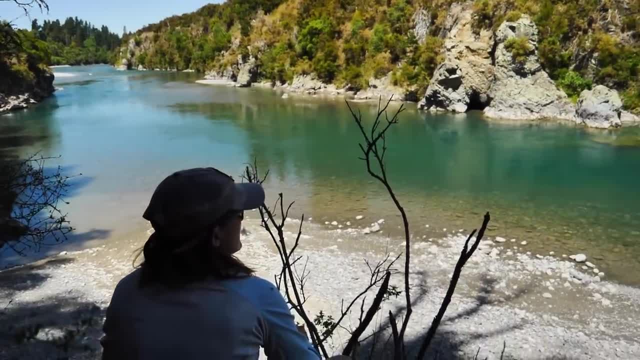 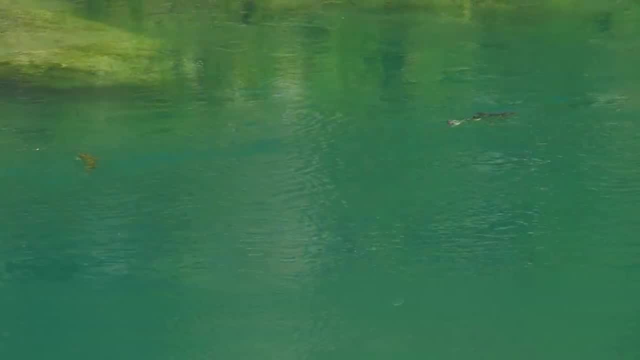 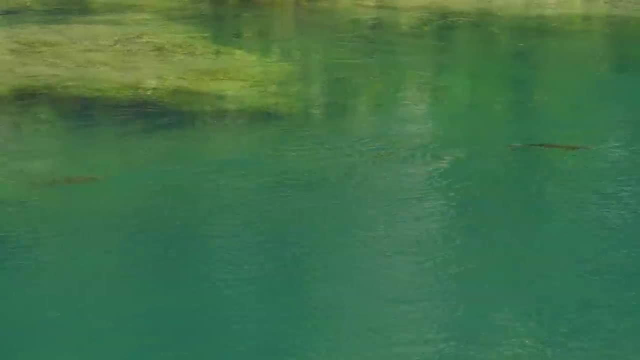 As we approached the tail out, glowing before us were two large browns in full display of an effortless feat. This is one of my most satisfying filming experiences. I climbed up on a rock face, keeping in the shadows Over 70 meters away, handheld and manual focus on the long lens. my initial anxiety was through the roof, but it soon ebbed to the rhythm of the concert before me. 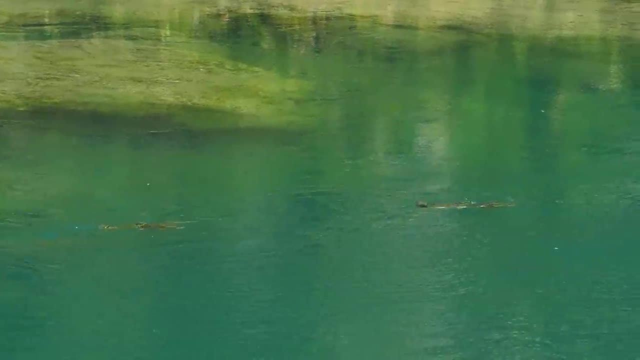 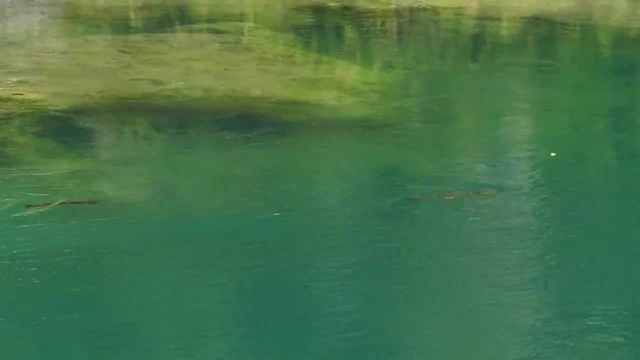 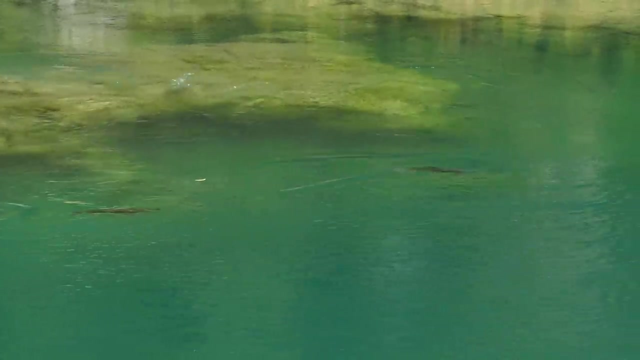 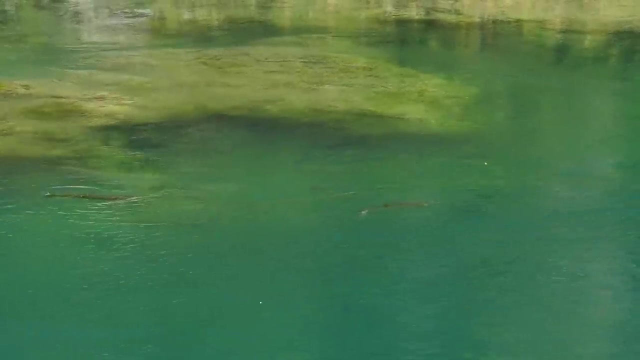 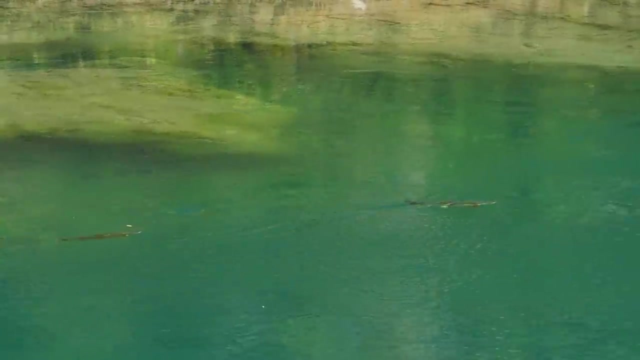 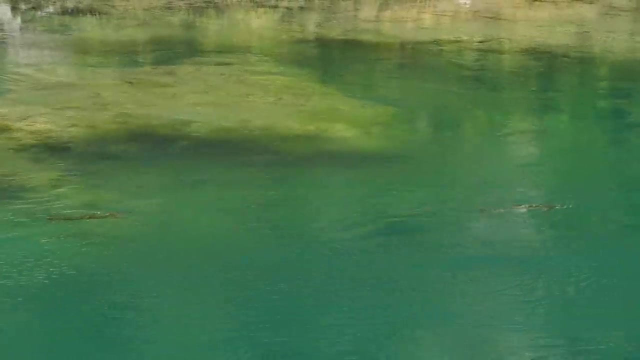 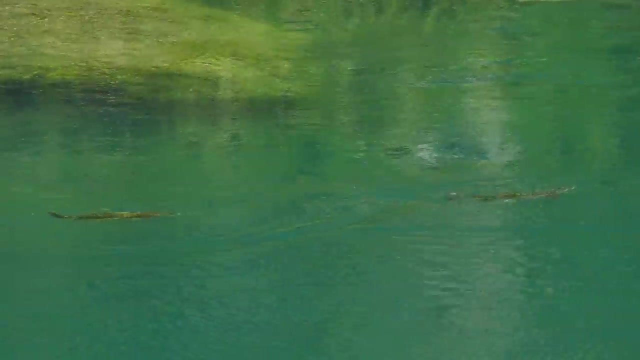 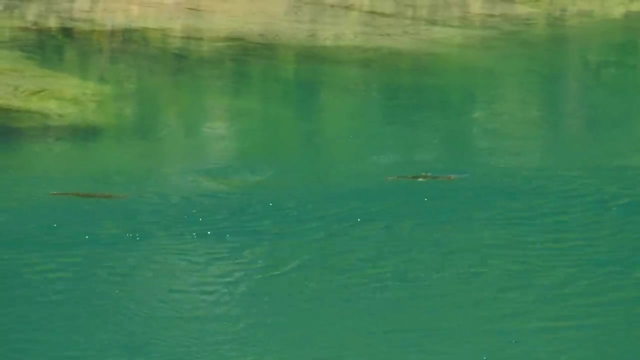 I climbed up on a rock face, keeping in the shadows. Over 70 meters away, handheld and manual focus on the long lens. my initial anxiety was through the roof, but it soon ebbed to the rhythm of the concert before me, Over 70 meters away, handheld and manual focus on the long lens. my initial anxiety was through the roof, but it soon ebbed to the rhythm of the concert before me. 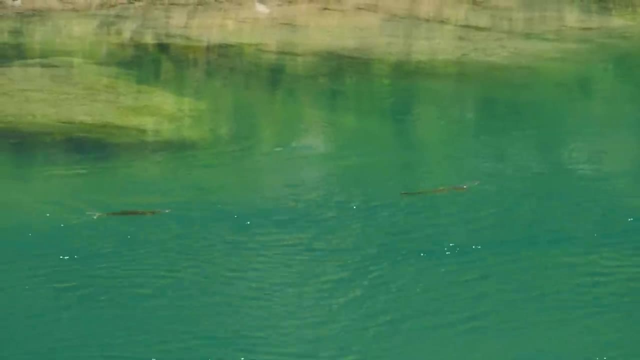 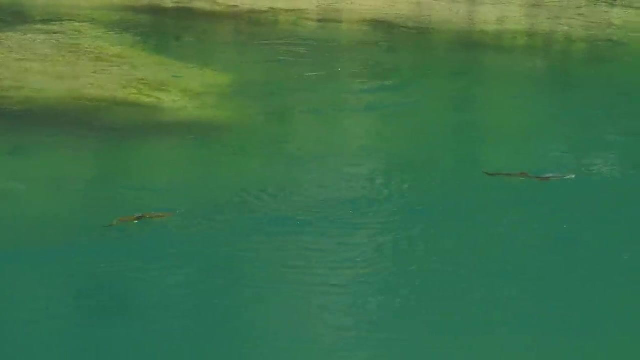 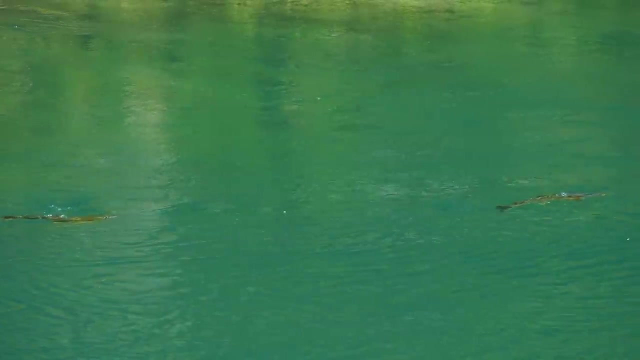 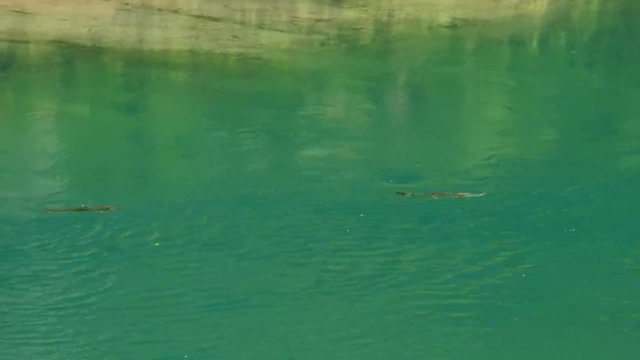 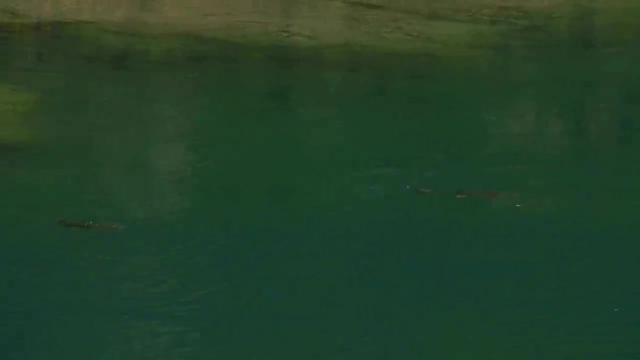 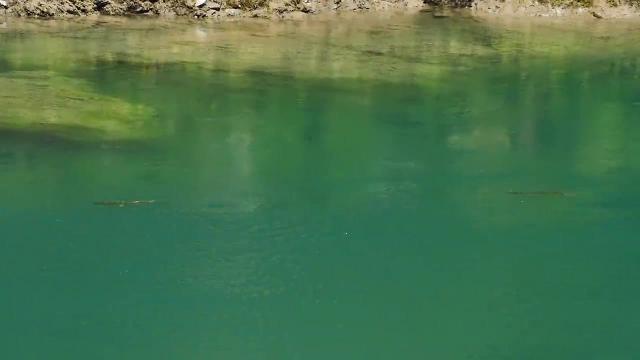 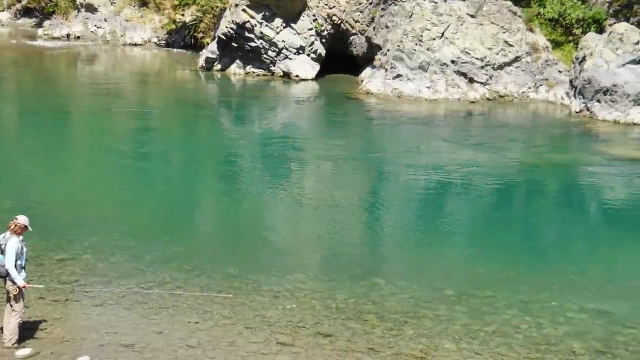 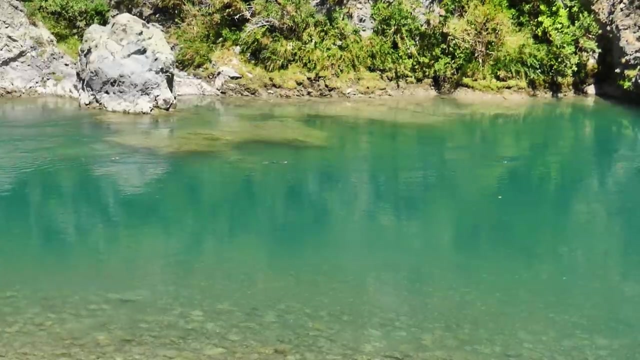 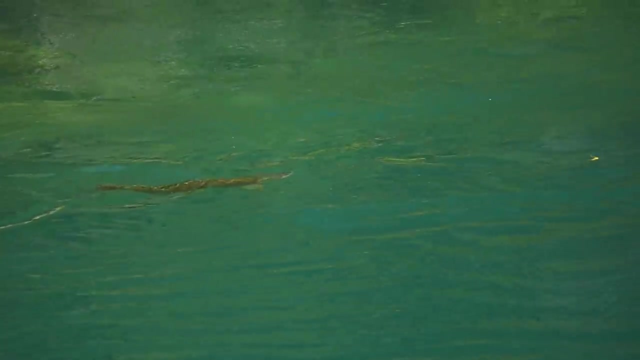 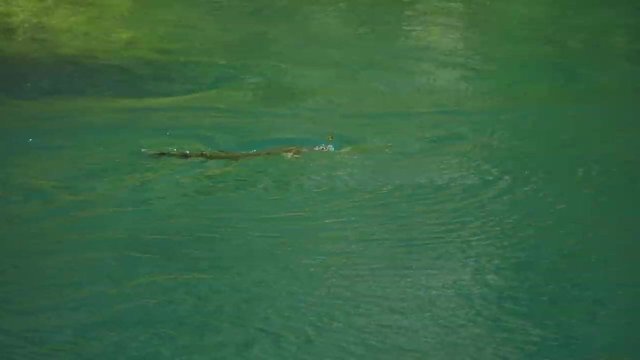 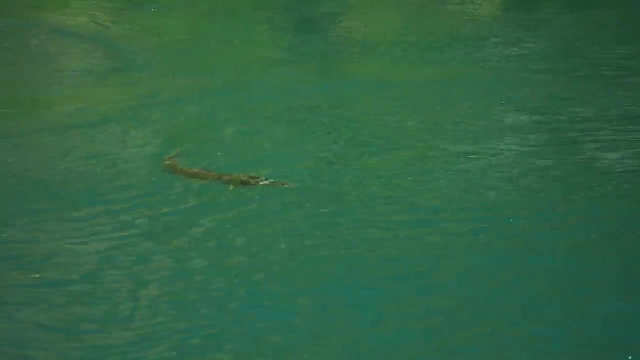 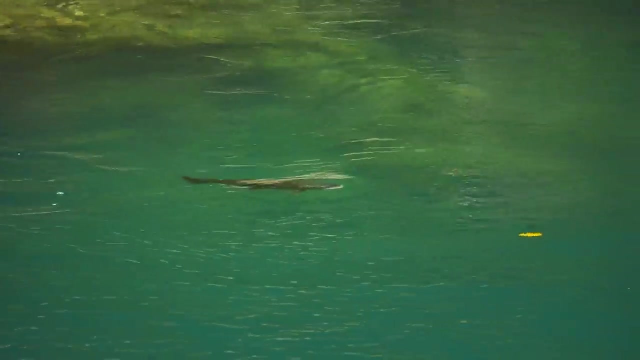 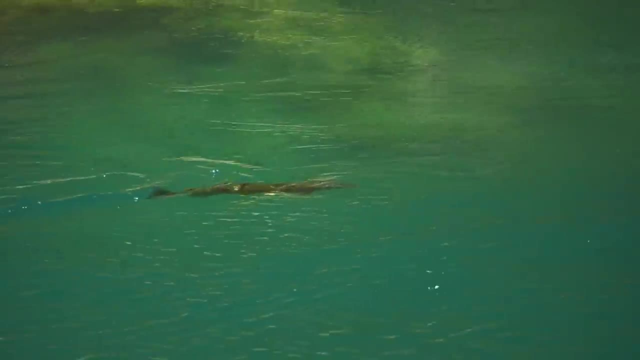 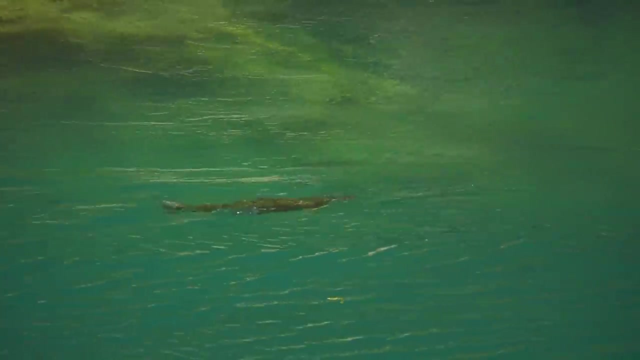 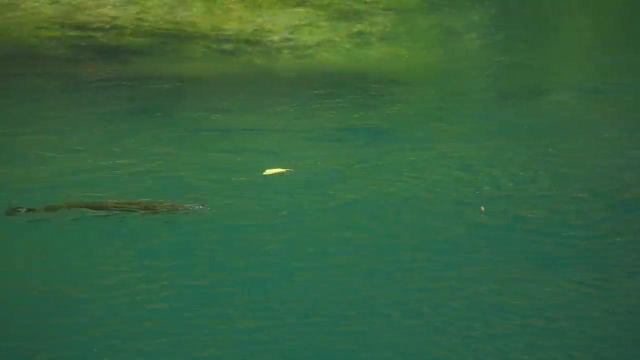 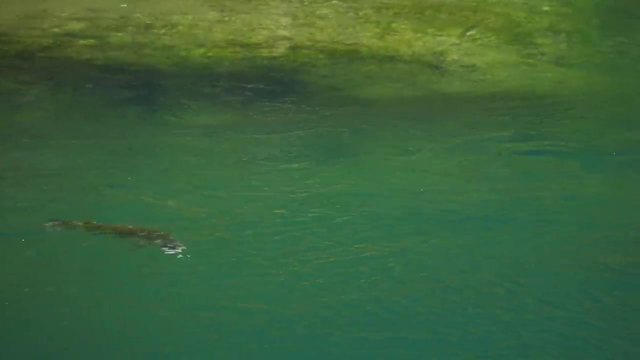 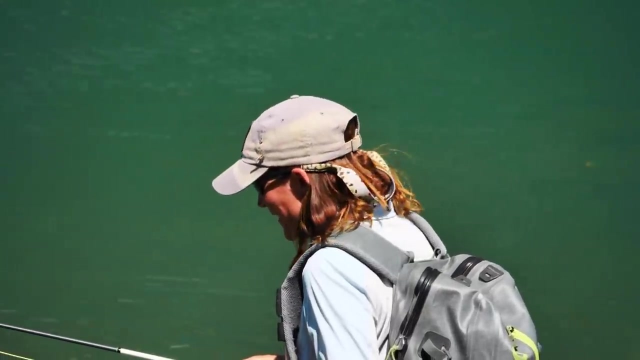 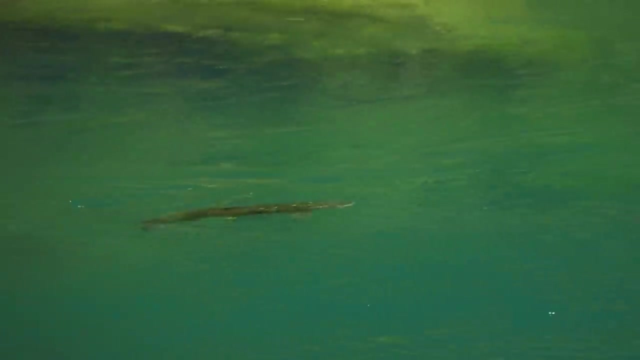 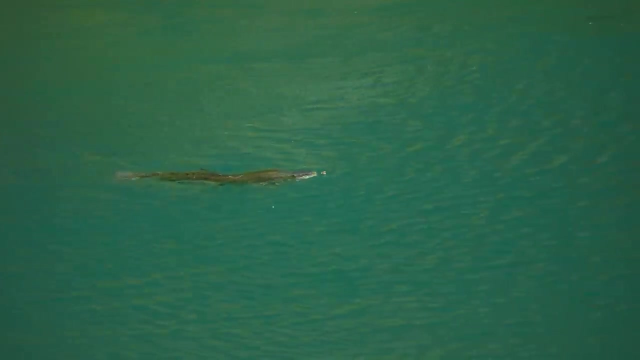 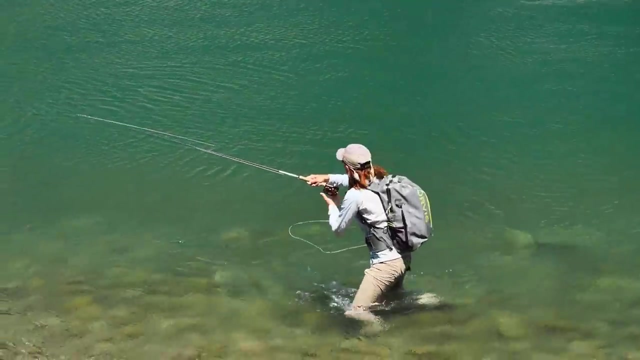 I flared out, but for Dave to call when they were two rods apart and had a go. As soon as I hooked up, I angled my rod down and steered it away from the big male upstream. I thought I had it under control and was horsing it over when it simply puffed. 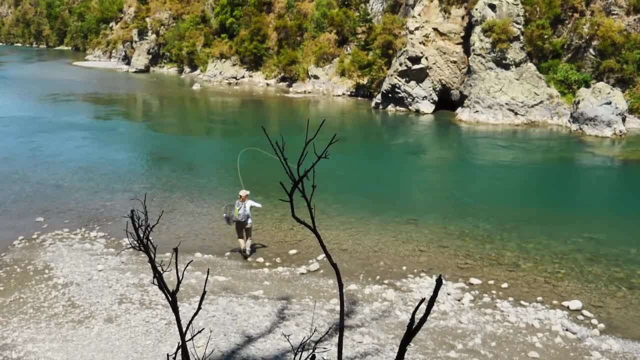 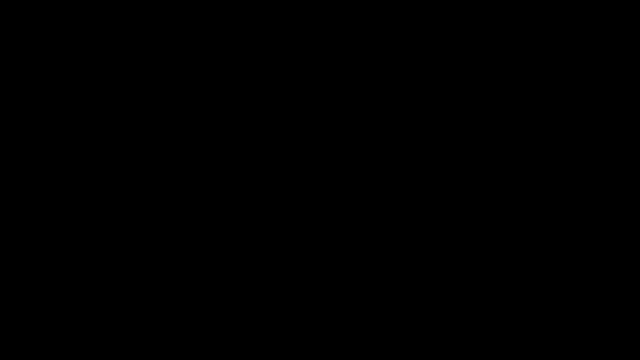 That distance of cast on a small dry is always a crapshoot. You bet I was gutted to drop that one. You bet I was gutted to drop that one. You bet I was gutted to drop that one. It was rough to drop that one. 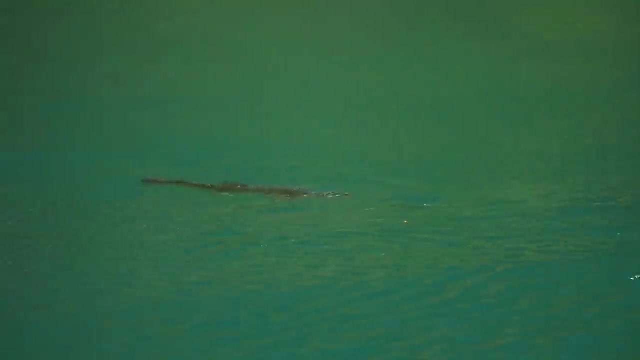 It was rough to drop that one, But there was still a stunner of a male popping mid-river. But there was still a stunner of a male popping mid-river. Given how it was feeding, I was gonna get an eat. 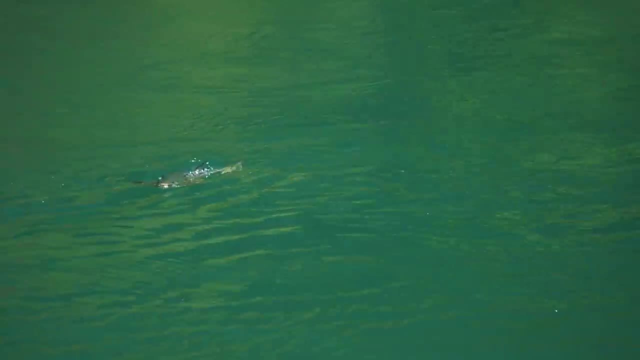 I couldn't lead it too much as to avoid a hooking drag on my near line, inducing a bad hook set, but I had to go at it. Lord, can you give me a little bit of grace? Oh, can you hear me? 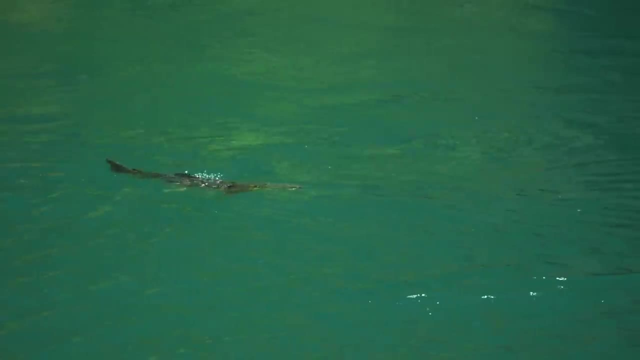 It's been one of those days, So I'll be waiting down by the riverbanks. You know I'll be praying, So please don't delay. Oh, please don't delay. Lord, can you give me a little bit of faith? I want to believe And I don't want to break. 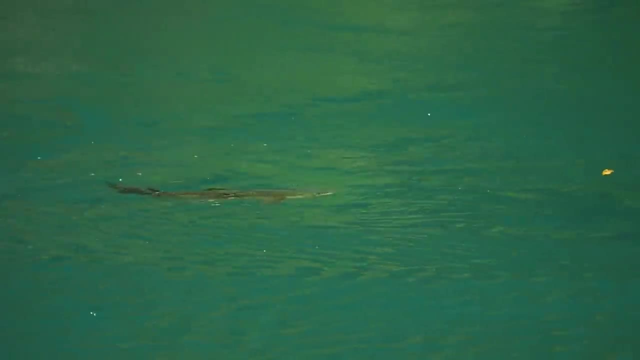 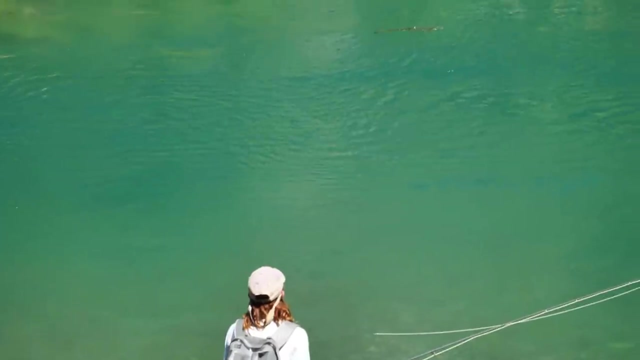 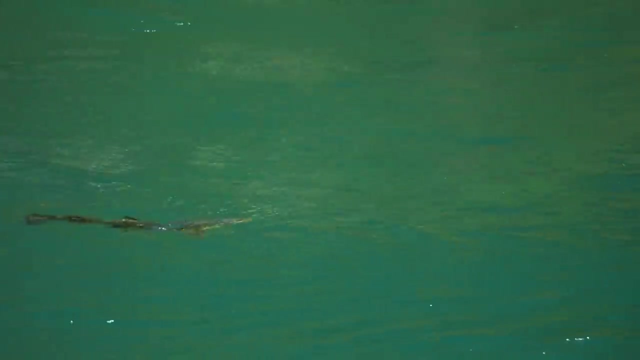 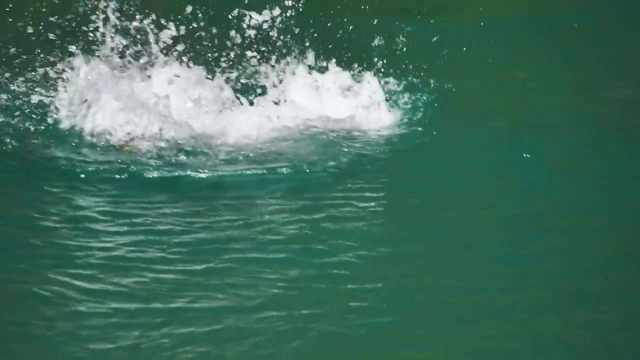 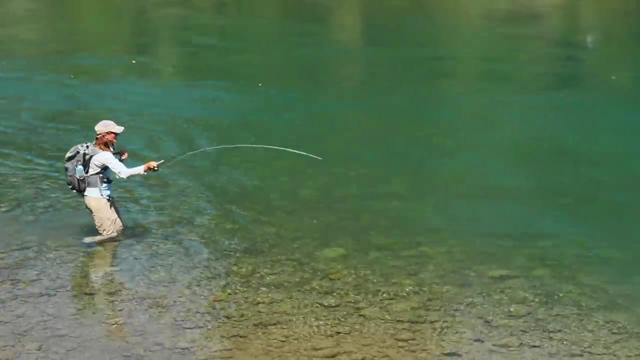 A moment of relief Would go a long way. You know I'll be praying, So please don't delay. Oh, please don't delay. Oh, please don't delay. Lord, can you give me a little bit of grace? Oh, please don't delay. Lord, can you give me a little bit of faith? 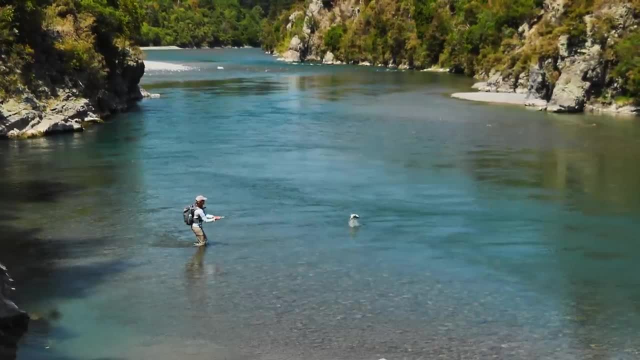 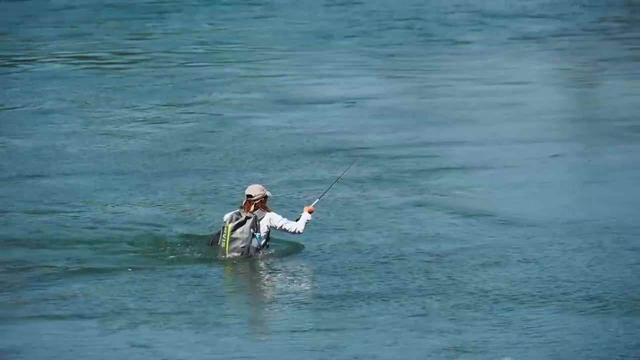 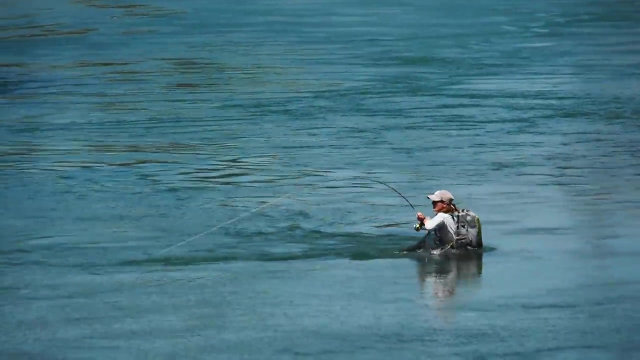 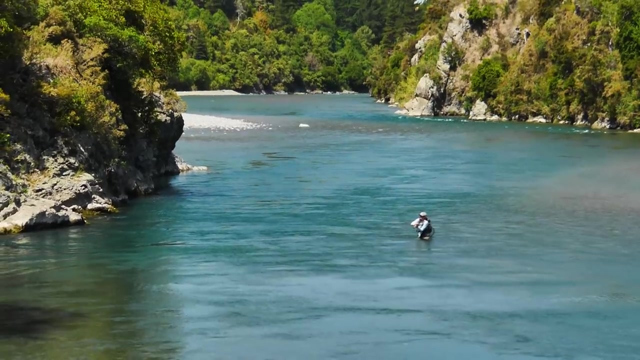 Oh, please don't delay. Show me There are days I come, and I I'll keep Me learning. Kneel it in the mud and show me Better days are coming, and so I'll keep. Kneel it in the mud and show me Better days are coming, and so I'll keep. 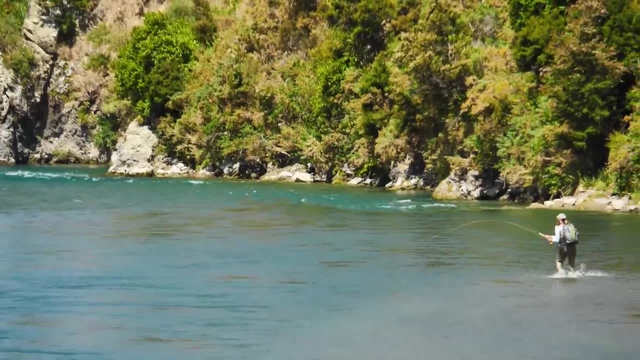 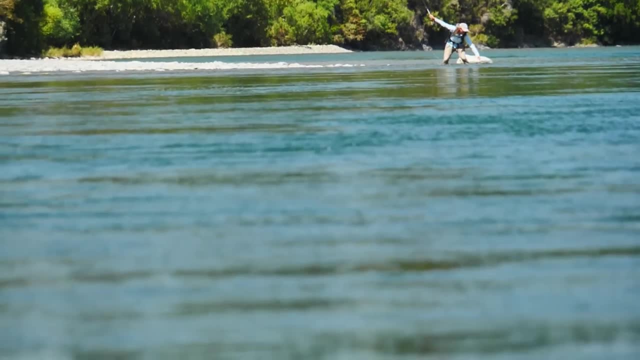 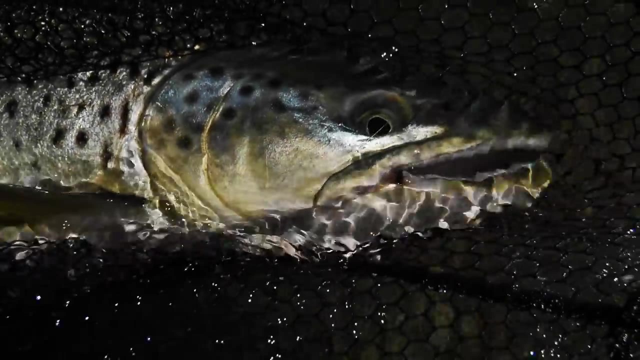 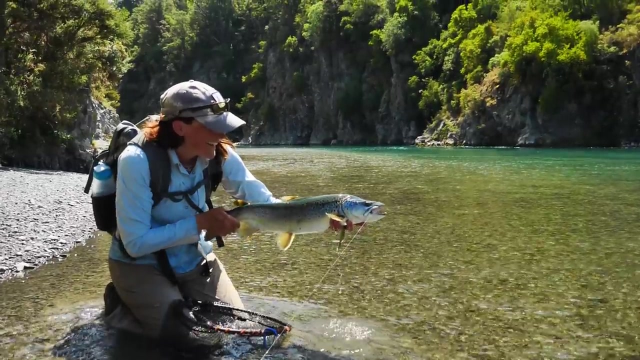 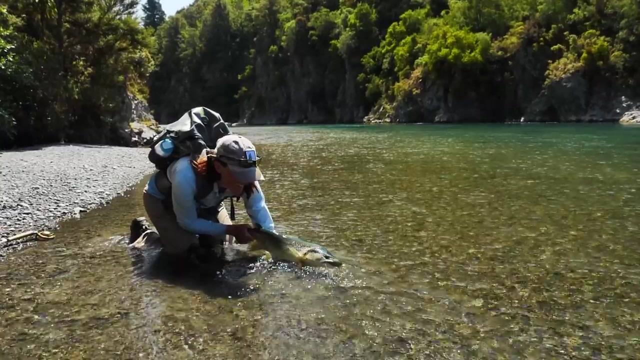 Lord, can you give me a whole lot of strength, Cause I keep reliving every single mistake. Oh, please, don't believe, Oh, please don't believe, Oh, please don't delay. You know, there's only a few times on a trip that you just get really epic moments. 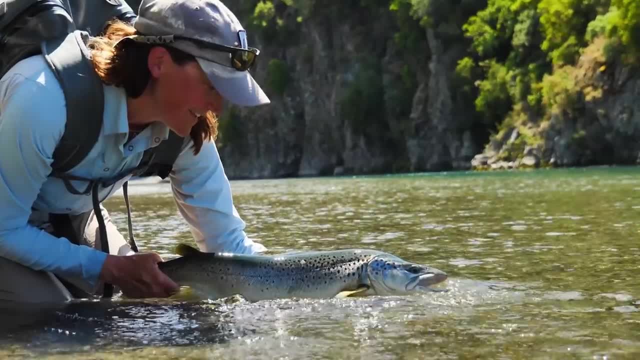 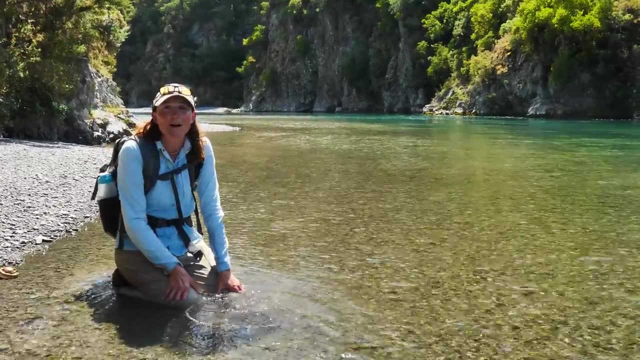 And that one was for me: epic. We didn't have much expectation coming into this day. We were dead tired and thought we gotta take it on. Look at this amazing sunny weather. It's so gorgeous out here. Cicadas are chirping and we're like, hey, we gotta go check out this river. 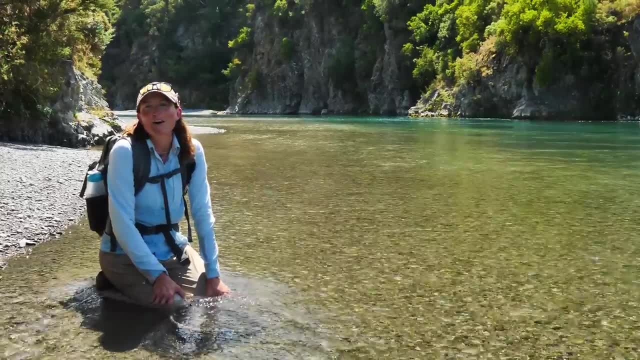 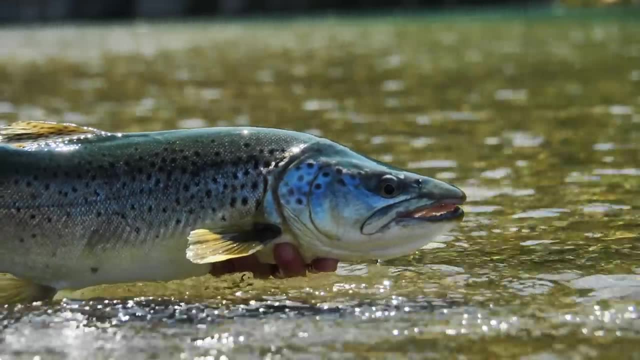 I didn't think we'd come across many fish, But anyway, we came across exactly what we'd been hoping for, Which was just rising fish, And there was two. they were like a rod length apart And Dave got on the camera And I think he had a whale of a time. 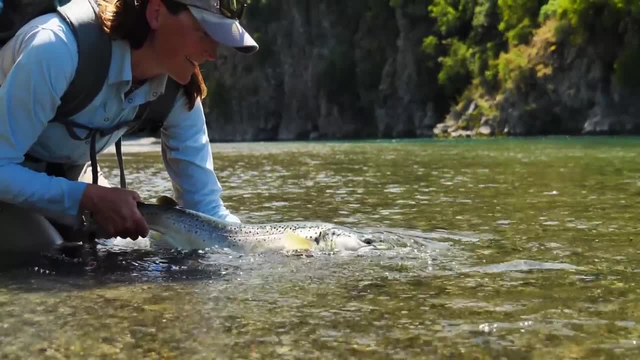 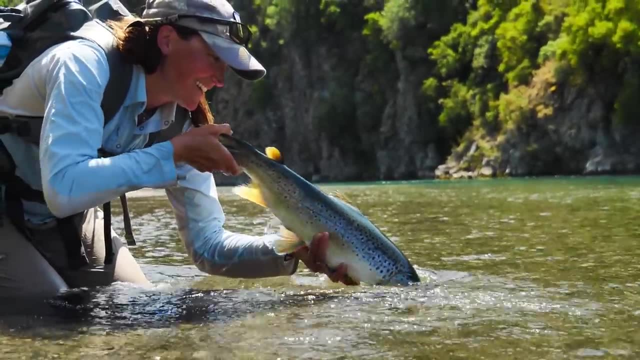 Filming them rising, And I hooked into the first one And brought it to shore And, just weird stroke of luck, It got off before I got it in the net. No big deal, it was the lower one. We knew it was a smaller fish, And so then 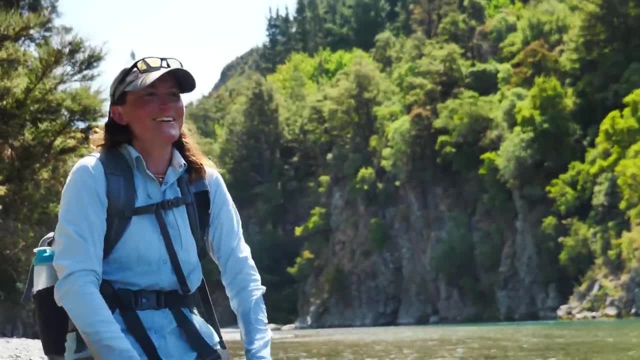 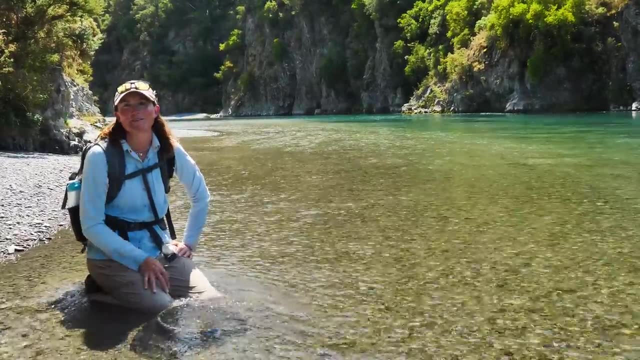 Dave was still up on the bank filming And he was happy doing that. So I went for the second one And it was this guy And man. they were just chomping, chomping on the surface Going to town. I mean even eating leaves. 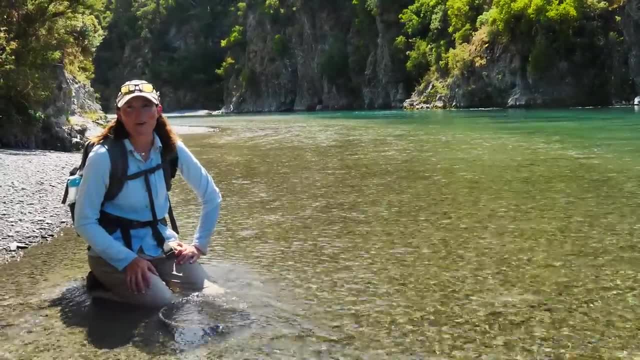 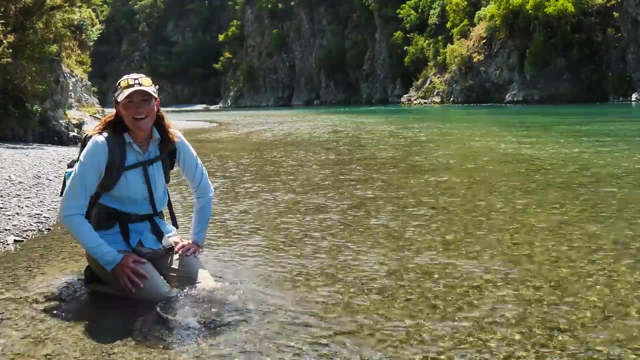 Anyway. so I was gonna get a take, no matter what, And I just put out this mayfly That Dave and I have designed together And tied quite a few, And he ate it, And it was just a gorgeous eat. And then the fly came out of the net. 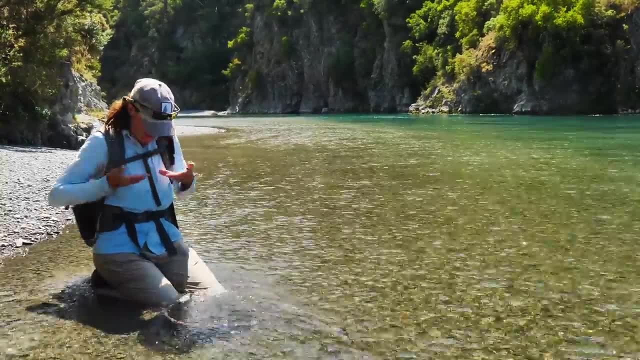 And I was like oh my gosh. And I was like oh my gosh And the fight had me worried Because, as you see, I was like Basically chest deep, Having to kind of get across the river Because this fish was going right into that. 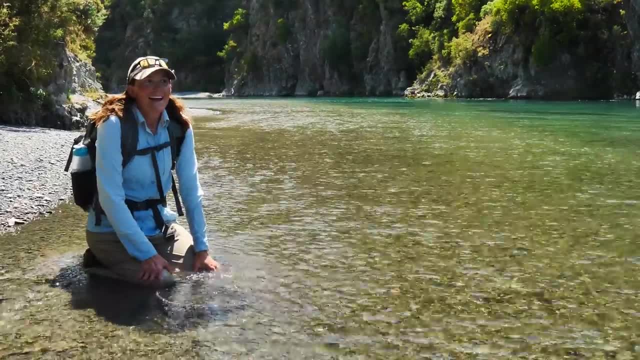 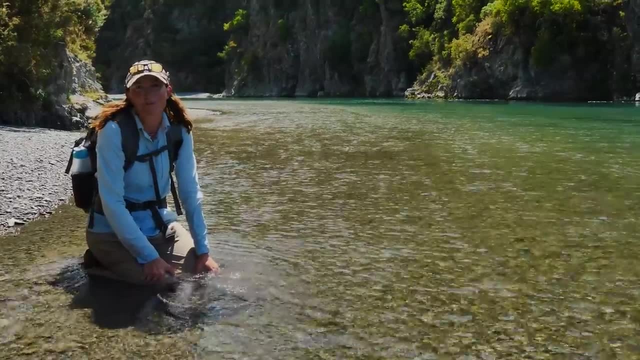 Big deep trough in the canyon wall And I got him Before he went down into the next set of rapids. So really wonderful, wonderful moment for me, Loved it. After that we were cliffed out by canyon walls, So there was only one thing left to do. 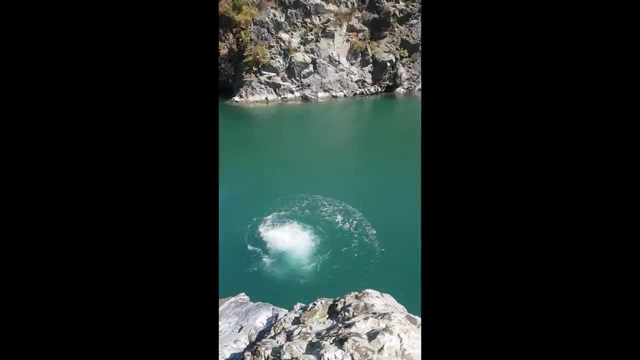 And that was To keep going up this way. Just put on our gear And stay at that base. You can't go up, right? So you're gonna have to do that. You can't go up or down, Just put your feet on the grass. You can't do anything. Just move your feet And don't move your feet, And just like that, And you're still hanging on And don't move the other side, And this thing keeps on coming And it's like I should try that, But I think it's the one thing That keeps me sticking theול. And it's something that I've always wanted to try, And it's something that I've always wanted to try- Like myself, I guess. But yeah, I think I'm gonna try that again and then we'll see. 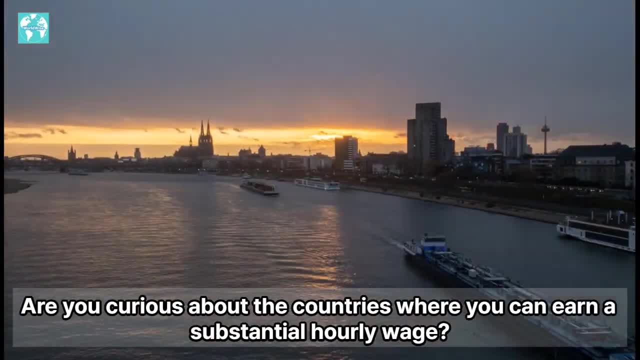 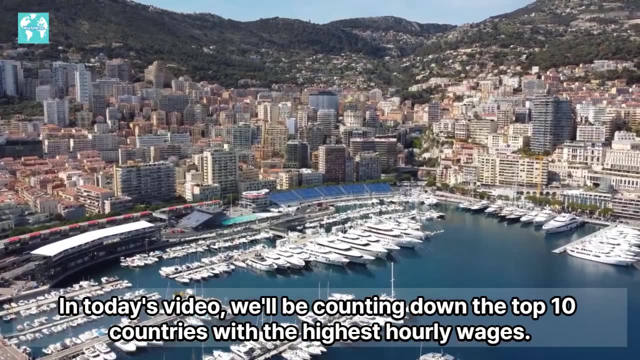 Hello money-minded viewers, Are you curious about the countries where you can earn a substantial hourly wage? Well, you're in luck. In today's video, we'll be counting down the top 10 countries with the highest hourly wages. So let's dive into our list, starting from number 10.. Number 10.. Ireland: Known for its thriving tech industry and favorable tax environment, Ireland offers attractive wages, particularly in the technology sector. Additionally, Ireland's stunning landscapes and rich cultural heritage make it an attractive destination for professionals seeking both financial rewards and a high quality of life. As of 1 January 2022, the national minimum